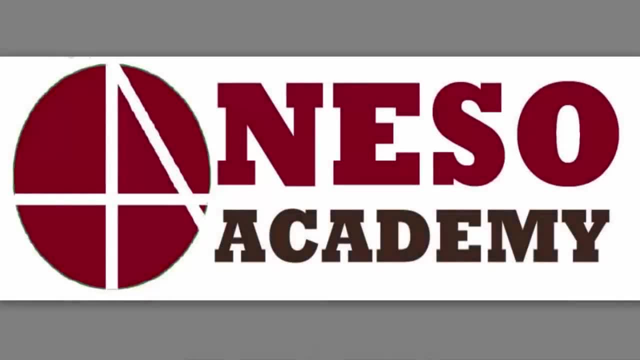 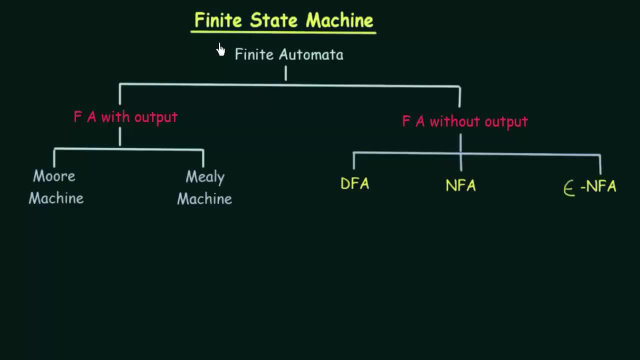 Hello everyone, welcome to the next lecture in theory of computation, and in this lecture we will be studying about finite state machines. Alright, so let's get started. So, finite state machines. it is also known as finite automata, and this finite automata is divided into two broad categories. 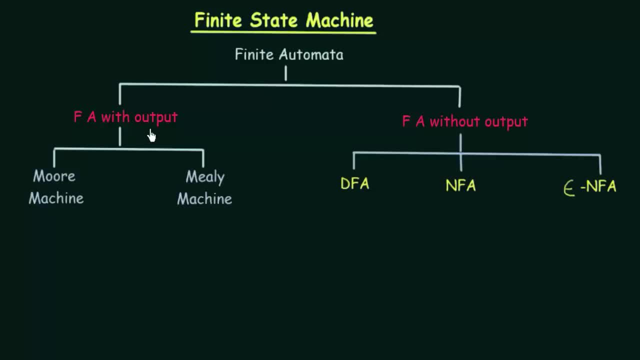 The first one being finite automata with output and the second one being finite automata without output And a finite automata with output. we have two categories, namely Moody machine and Mille machine, And in finite automata without output, we have three categories, namely Deterministic Finite Autometer or DFA. 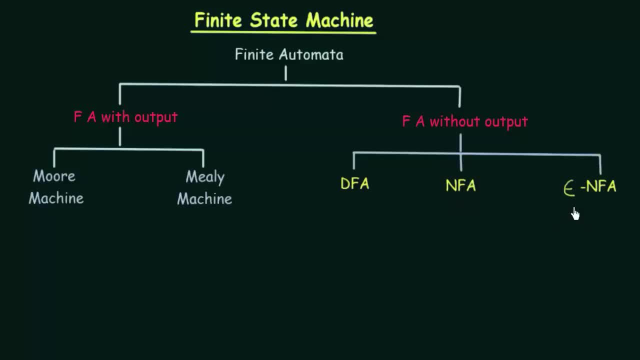 Non deterministic finite automata, or NFA, and Epsilon. Non Deterministic finite Automata or Epsilon, NFA. Alright, so in this lecture we will be mainly focusing and studying about Deterministic finite automata, or DFA. Okay, so DFA it stands for deterministic finite automata. 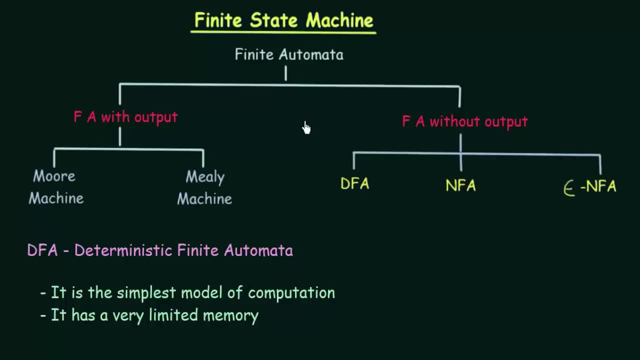 Before we start off with DFA, Let us remember two important properties of finite state machines that we should always remember, and they are finite state machines. it is the simplest model of computation and Also, finite state machines has a very limited memory. So these are two important points that we should always keep in mind before we 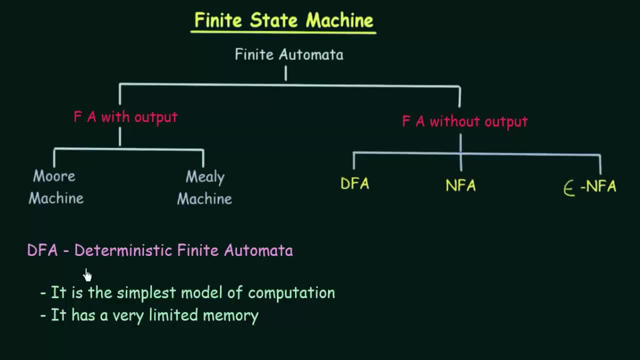 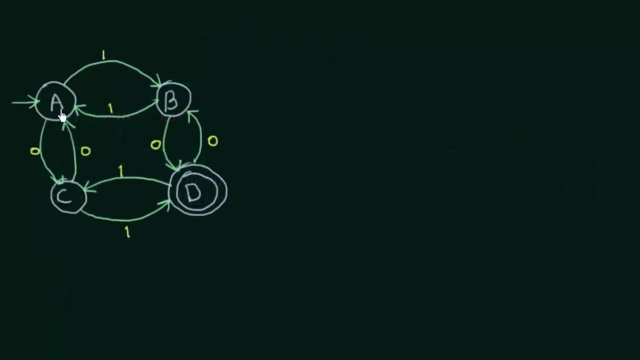 Study anything related to finite state machines. Okay, Now we can start off with deterministic finite automata, or DFA. now, to make DFA clear, Let us take a simple diagram that will make the structure of DFA clear to us. So this diagram here: it shows us the structure of our deterministic finite automata, or DFA. 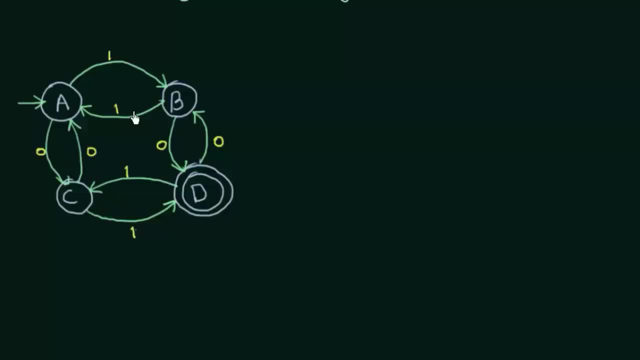 So first, when you look at this diagram, You may Feel confused. what are these? what do we see here? We see some circles labeled as ABCD, we see some edges, some arrows pointing here and there, and we have seen some Labelings like one one, zero, zero, one one. and what are all this? 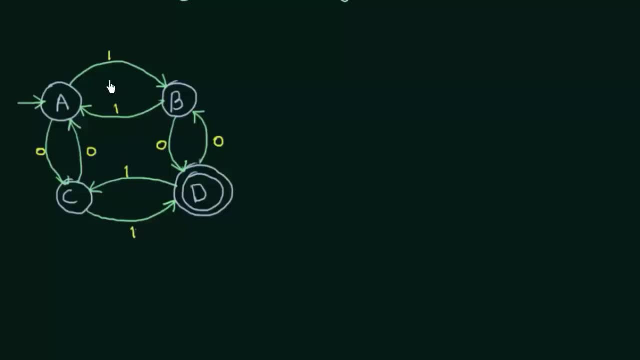 Okay, so I will explain to you what this means, So that the structure of this DFA becomes clear to us. So, first of all, The first thing that we need to know are states, these circles Represented by a, B, C and D. these circles are known as states. 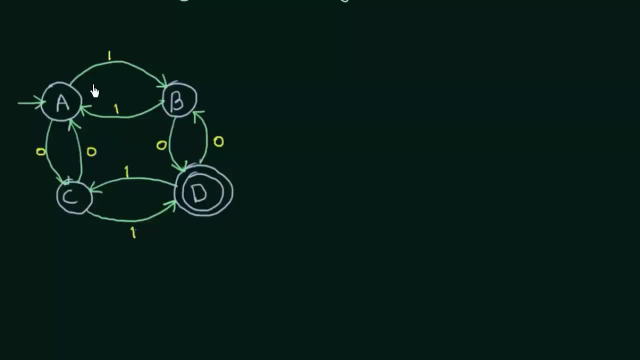 Okay, a, B, C, D are states. and then we see some edges. see, one edge goes from A to B, another edge goes from B to A, and here also we see an edge going from A to C and another from C to A, and here we see one going from C to D and from D to C. 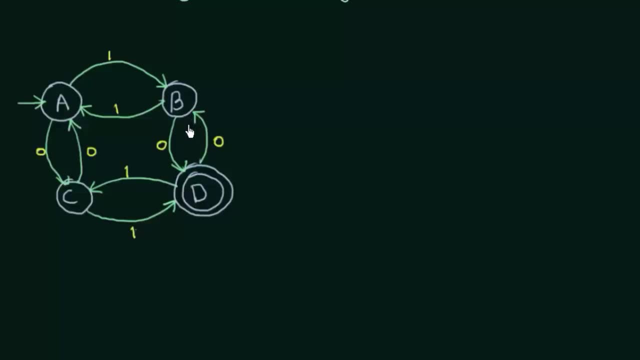 B to D, D to D. So what are these? these edges are actually the transitions. so what does this mean? this transition means that, suppose we are in state a and this edge Labeled with one. this labeling of edges are known as inputs. These are our inputs. 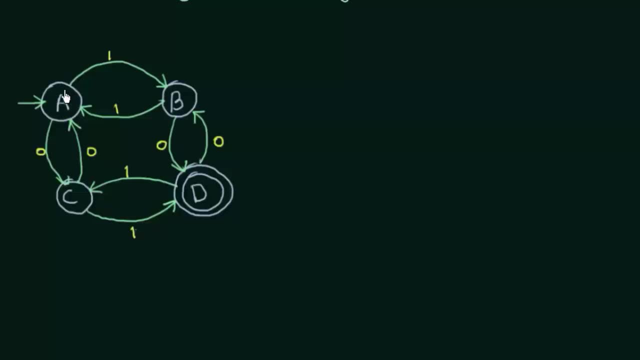 so it. what it means is that when I am in state a and if I get input one, if the input I get is one, so my state a goes from A to B, All right. and in the same way, if I am in state a and if I get input zero, then what happens? state a goes from A to C. 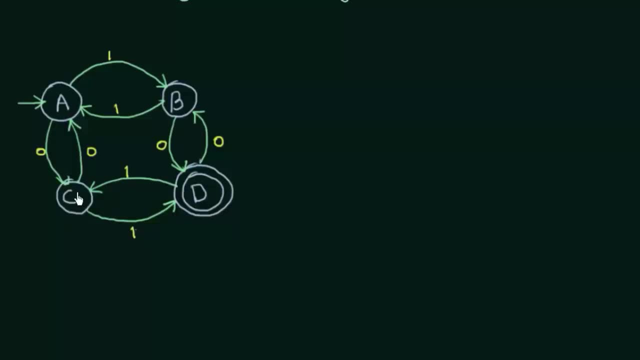 Okay, and let's take one more example. Suppose I am in state C and I get input one. So where do I go? I go from C to D, and in D, if I get input say zero, it goes from D to B. so that is how the 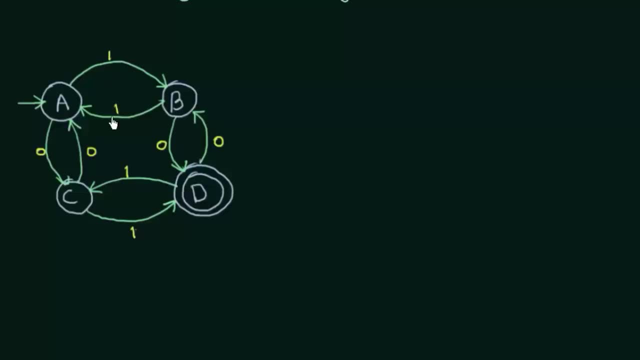 Transition occurs. so this labelings of the edges- They are our inputs and the circles are our states. so it shows how the states transits from one State to another on getting certain inputs. Okay, so that was about the states and the inputs. Now we see that there is something different about state a and state D. 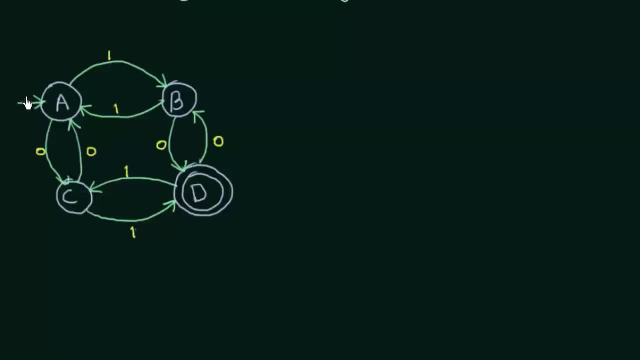 So what are they? in state a, we see an arrow that is coming from nowhere and pointing To a. so what is this? this means that A is the starting state or the initial state of this DFA. whenever you see an arrow coming from nowhere pointing to a state, that shows that that is the initial state or the. 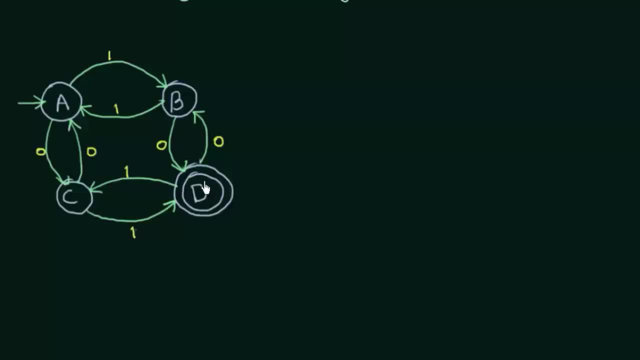 starting state and If you look at state D, there is something different. What is that? Every other states have one circle, but this state D has two circles. It has a double circle around it, and What does that mean whenever you see a double circle? 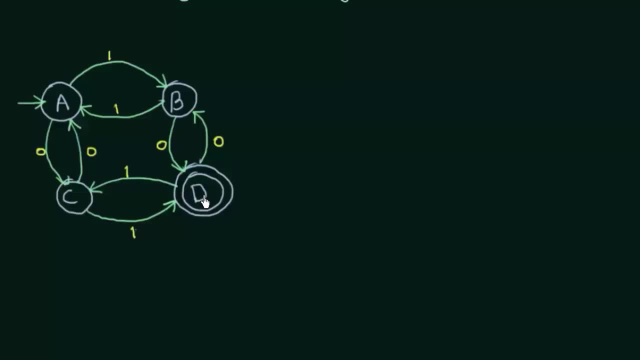 It means that that is the final state or the terminating state. So this state D, represented by two circles, It is the final state of this DFA. Alright, so those were the main things that you need to know about a DFA. so that makes the structure of DFA clear to us. 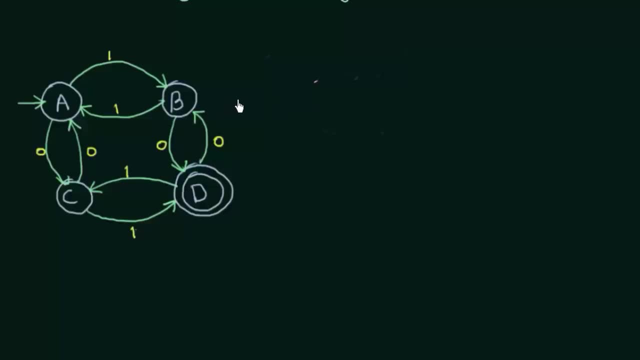 Okay, So now let us write down the formal definition of this DFA. so every DFA can be defined using five tuples, which are Q, Sigma, Q, naught, F and del. Every DFA can be defined using these five tuples. Now Let us see what are these tuples? What do they mean? 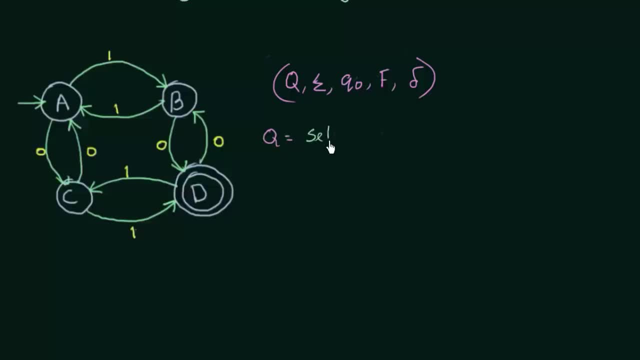 first of all, we have Q. Q is the Set of all States. the set of all states is known as Q. and what is Sigma? Sigma is the Inputs. our inputs is represented by Sigma. and then the next one is Q- naught. What is Q naught? Q naught is the. 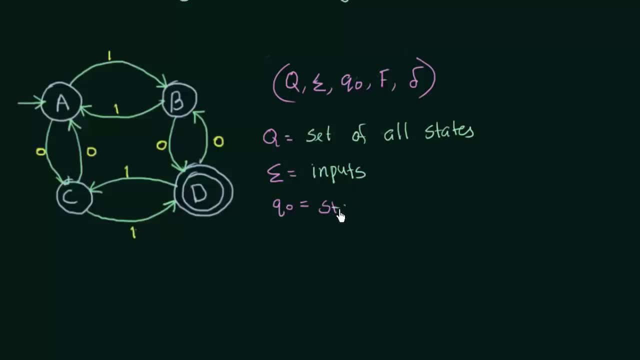 Start state, Start state, or it's also known as the initial state. It is an initial state, Okay, and then the next one is F. F is a set of. F is a set of Set of Set of Final states, Final states. The set of final states is known as F. so here, in this example, 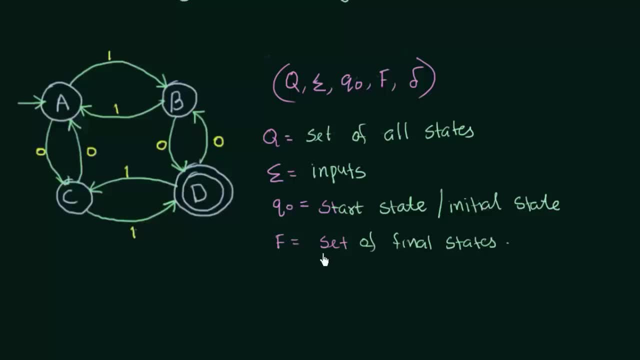 We had only one final state, but we could even have more than one final states, So that is why I have written set of final states. All right, and the last one is del. So what is del? del is a Transition function. it is a transition function. 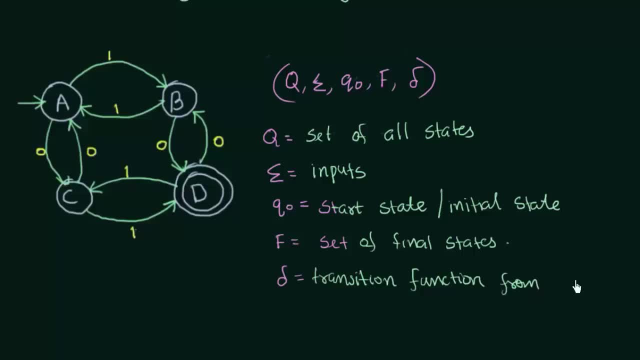 that maps, Okay, from Q cross Sigma to Q. it is a transition function that maps Q cross Sigma to Q. don't worry, Even if I don't understand this, this will become clear when I take the example I will be showing you in the example. Okay, so 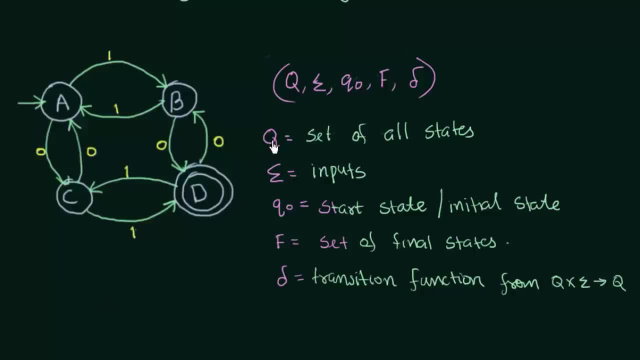 Now let us try to write down What are the values for these five tuples for this example that we have taken here for our particular DFA. What are the values for this Tuples? first of all, we have Q. So what is Q here? Q is a set of all states. So what are the set of all states a, B, C and D? a. 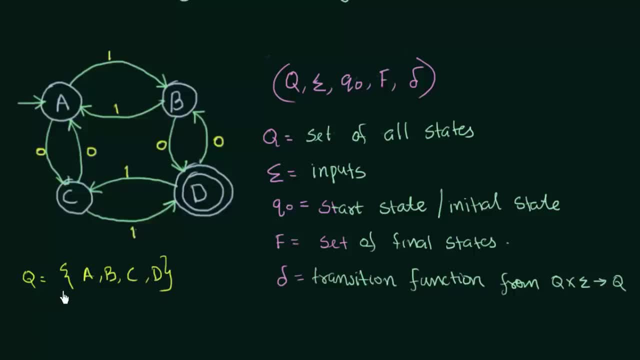 B, C and D. This is our Q, and what is our Sigma? Sigma is the inputs. What are our inputs? We have inputs here: 0 and 1 zeros, and ones are the inputs we use here. So it is 0 and 1, okay, so. 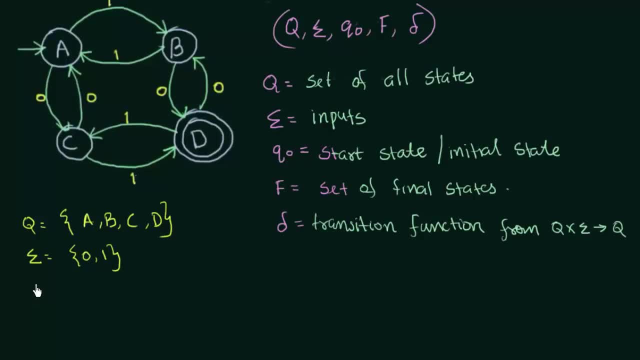 that is a Sigma. and what is the next one? Q naught. Q naught is the start state or the initial state. So I already told you, whenever we see an arrow coming from nowhere pointing to a state, that is the start state. so our start state here is a. 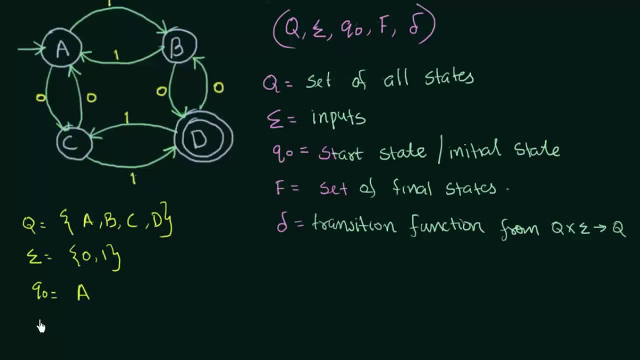 a okay, and then the next one is F. F is the set of Final states. So what is the final state here? D? We have only one final state. whenever you see a double circle, that represents a final state, So I should probably put it in a bracket because it could be more than one. 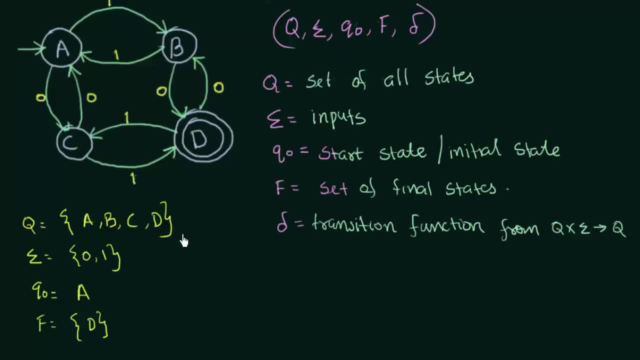 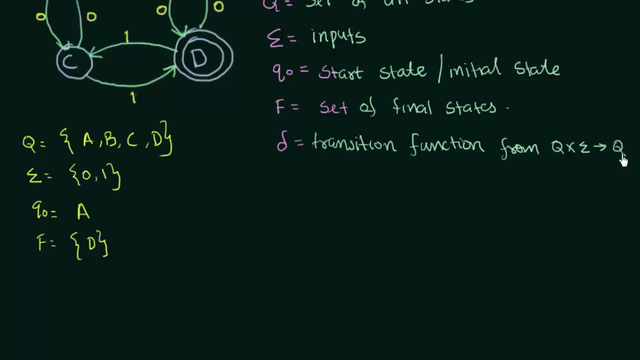 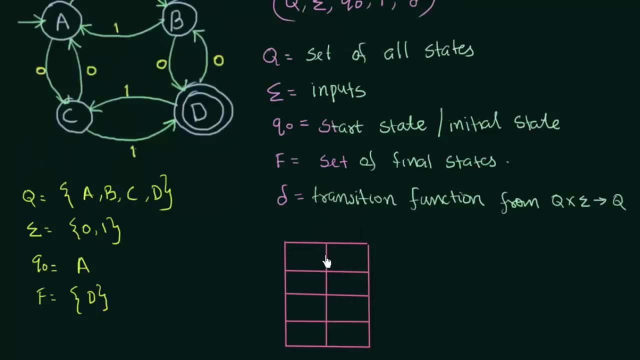 But in this example it is only one so set. our set of final state is D, and then the last one, Del. del is a transition function from Q cross Sigma to Q. now to Demonstrate this, let me take a table over here. I'll use this table to explain what is. 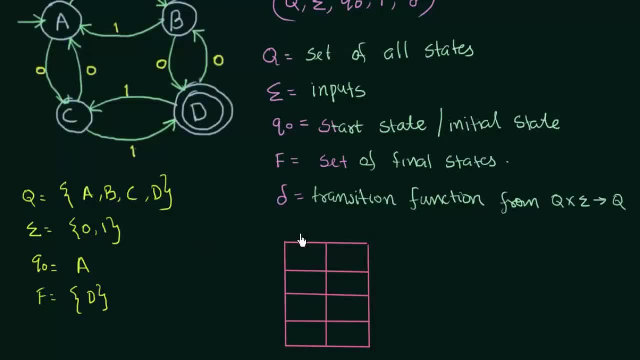 Del. so for that, Let me have this table Where this top part will be my input: 0, 1, and I'll have my states in this part: a, B, C and D. Alright, now let's see What is this. What does this mean? 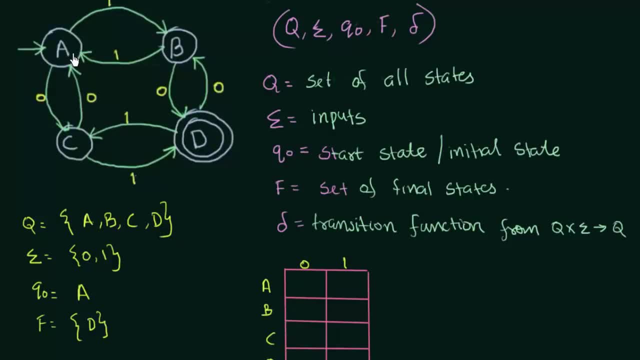 so Suppose I am in state a and I get input 0. So what happens? when I am in state a and I get input 0, it goes to state C. right a to C, I mean state a. if I get input 0, I come to state C.